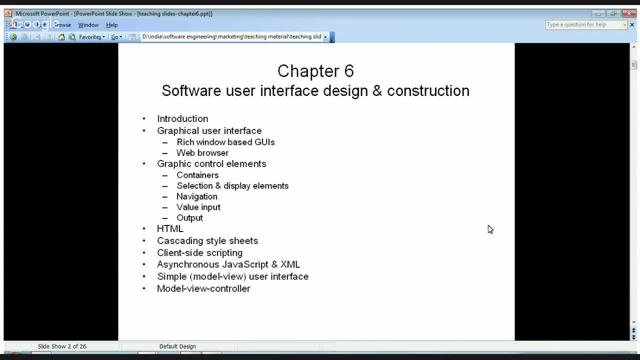 rich window based graphical user interfaces or GUIs of a browser, graphical control elements like containers, selections and display elements, navigation, value input, output, and then we will learn about HTML. then cascading style sheets, then client side scripting and then Ajax technology, which is used for sitting on your browser, is given for using google asssync from a browser. javascript leveraging xml will be used to comparable air dc file block that, considering all the events that will take place in this critical sad, I will only give a mentioned. 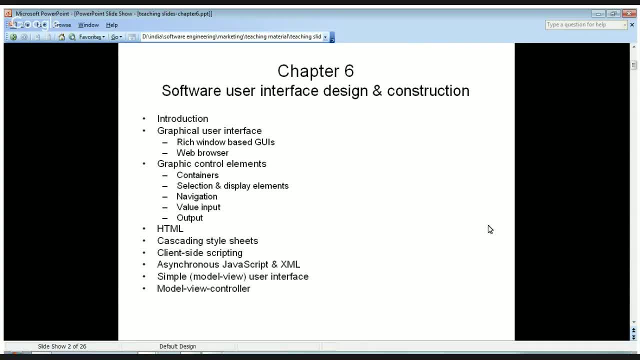 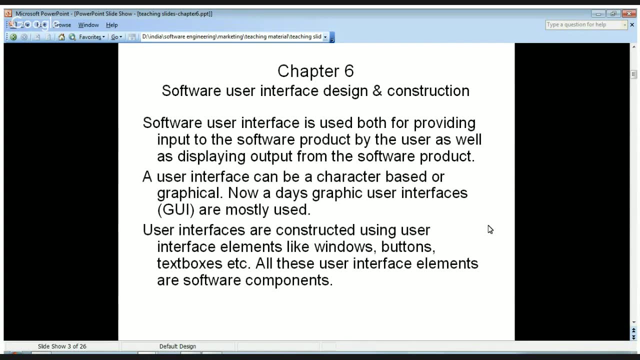 given a certain class in our example lenu, for javascript early, a sub s interface through which a user uses a software product, so he will provide some input and then the product will do some computing processing and then will come out with some output which will be displayed on the user interface. 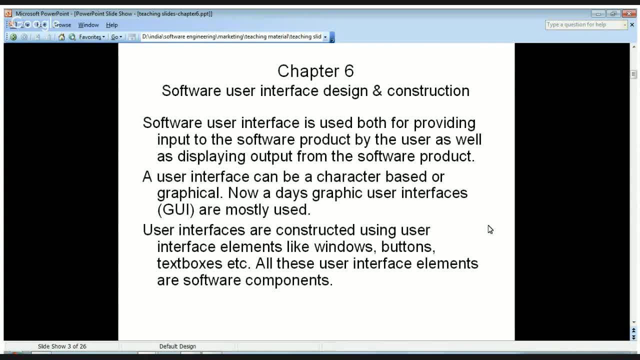 User interface can be character based or graphical. earlier we used to have character based user interfaces where the only way the computer output can be displayed was through characters on a screen, like in the days of the IBM supercomputers, or even in the client server. early days they 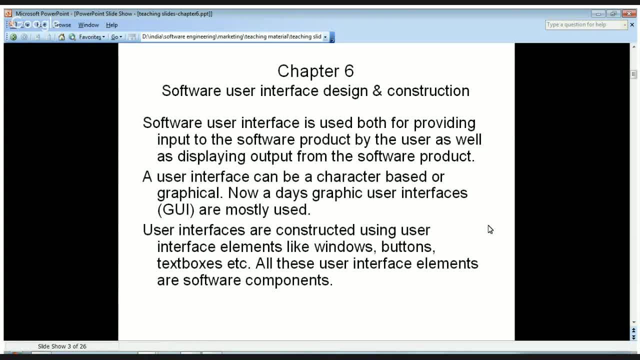 used to have only character based, But now we have graphical user interfaces Which are used mostly. So actually for graphical user interface you need a lot of processing power. Earlier computers never used to have this kind of processing power to have graphical user interfaces. but now a days even very small computers or even mobile handsets have good 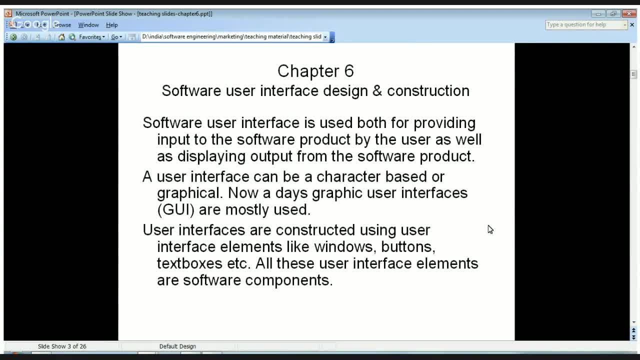 processing power, like they have very high capabilities- CPUs and memory cards, and they can display any kind of graphics, even 3D graphics, or even they can display videos. they can display, they can display 3D graphics, etc. User interfaces are constructed using user interface elements like windows buttons, text. 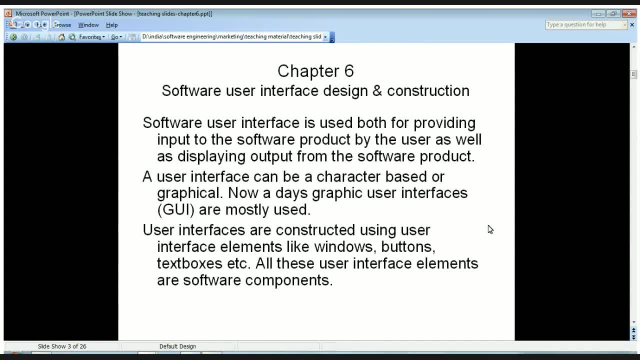 boxes, etc. All these user interface elements are software components. So most of the components for user interface are already built and you do not need to build these components. In very special cases, when the commonly available user interface elements will not serve the purpose for you, then you need to build a very specific user interface. 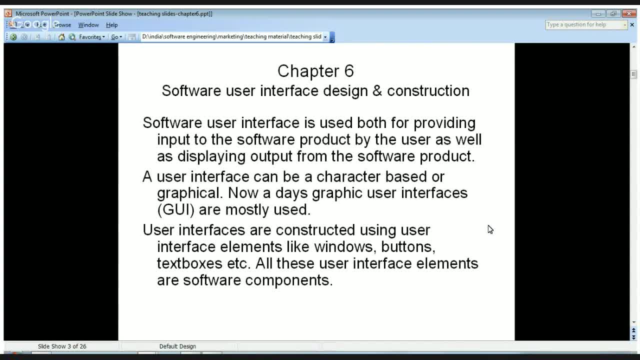 So that's the main thing. You need to use the interface control element, otherwise you already have them, so no need to build them. They are available in most of the development environments, like even for java, development environments like the one which is known as netbeans, provided by oracle or javascript. 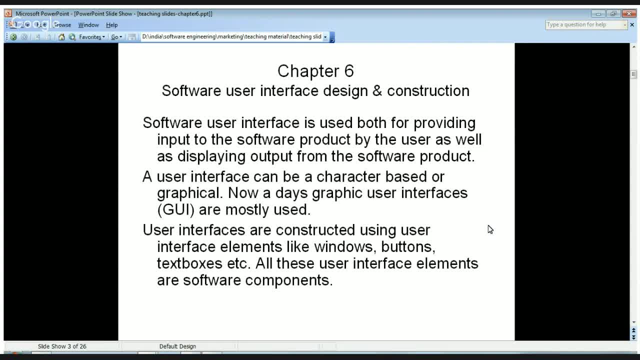 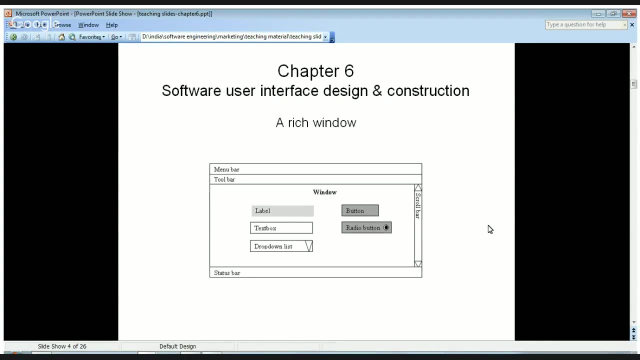 Some other companies are also providing so, similarly for some other vendors. you always have these development environments where the graphical user element controls are already built in the programming language. So one of the elements is the user interface. So the user interface, One of the important consideration in user interface, graphical user interface, like for 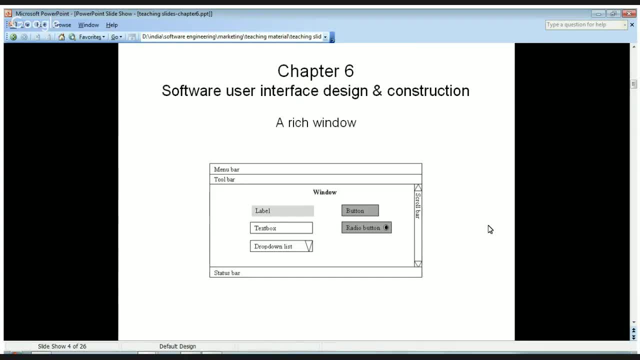 example, when you need to create a client server application- the client part- there will be a rich window. A rich window, like displayed here, has parts like the menu bar, the toolbar and the main window part, the body part Inside that you can have elements like labels and so on. 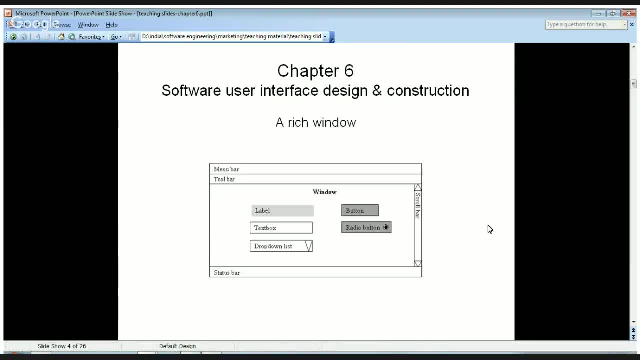 So this is the main part. So this is the main part. So this is the main part. You can have elements like the buttons, text boxes, et cetera. At the bottom of the window is a status bar, and then you also can have a scroll bar. so 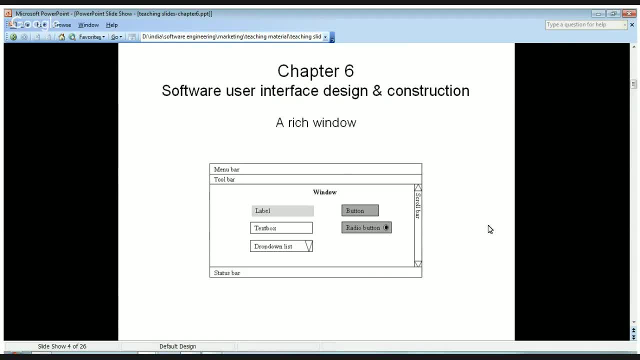 you can scroll through the window and then, for web based software products, you will have web browser window In. the web browser window is very similar to a rich browser, similar to a rich window, but it will have a universal resource locator bar where you need to provide the website or web page name and then it will browse. 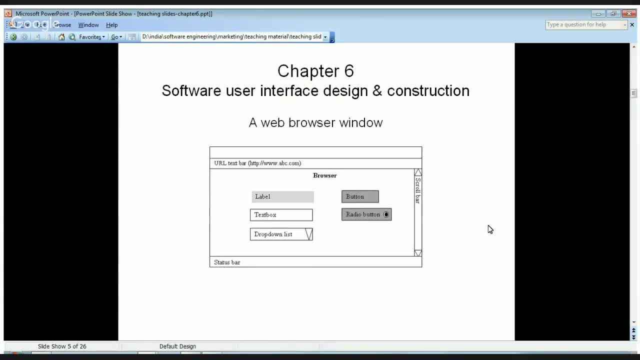 your browser will browse to that page or site and inside a web browser window you will have the same kind of user elements like buttons, labels, text boxes etc. and at the bottom of the window is the status bar. in the status bar you can display information like some operation is complete or some, if there is some. 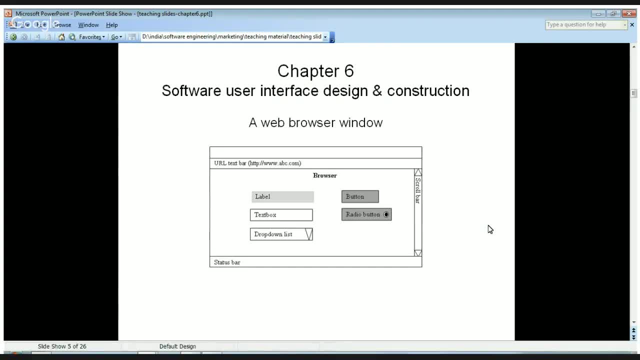 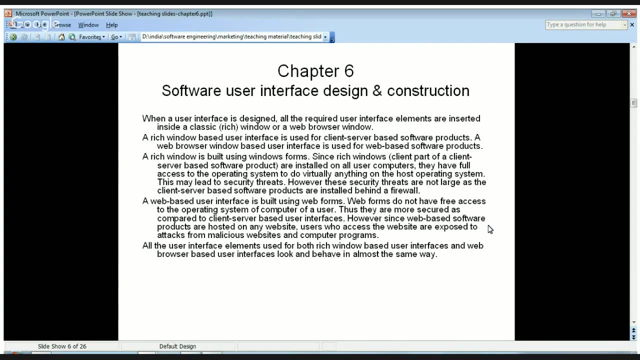 problem in the operation. it can be displayed in the status bar and again on the right side you will have a score bar so you can scroll through the window. when a user interface is designed, all the required user interface elements are inserted inside a classical dish window or a web browser window, a rich window. 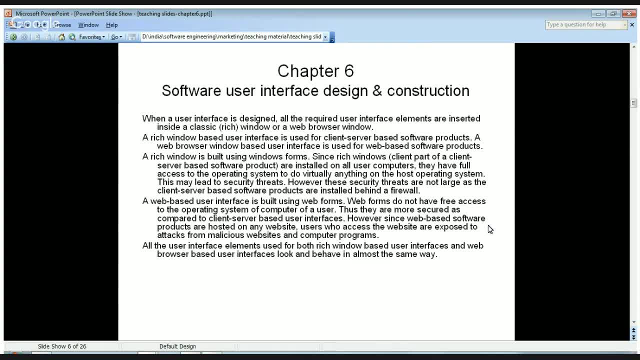 based user interface is used for client server based software products. every browser window based user interface is used for web-based software products. a rich window is built using windows forms. since rich windows- client part of a client server based software product- are installed on all these computers, they have full access to the operating system to do virtually anything on. 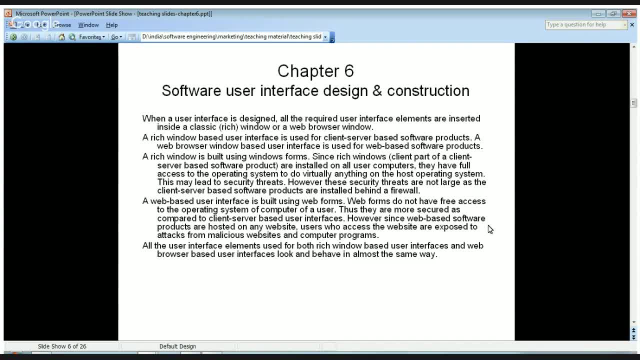 the most operating system. this may lead to security threats. however, these security threats are not large as the client server based software products are installed behind them- fireball. so this is important consideration when you you are building a client server software product and you are building the client part, so the client part will be rich windows and 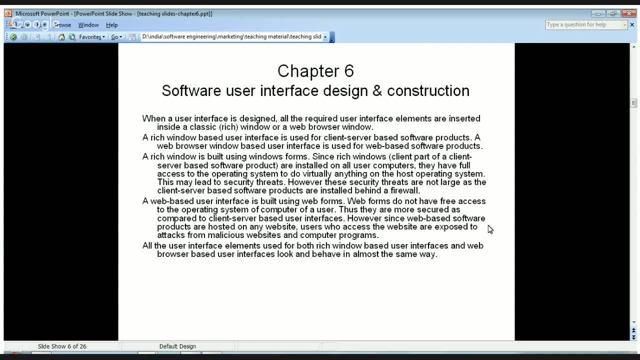 the, the controls and the window itself will have access to the operating system on which it is installed, because, uh, it is directly installed on the uh, on the operating system of your computer, so it can have access to everything on the on your computer. it can access a file, it can modify your file or you can delete a file. it. 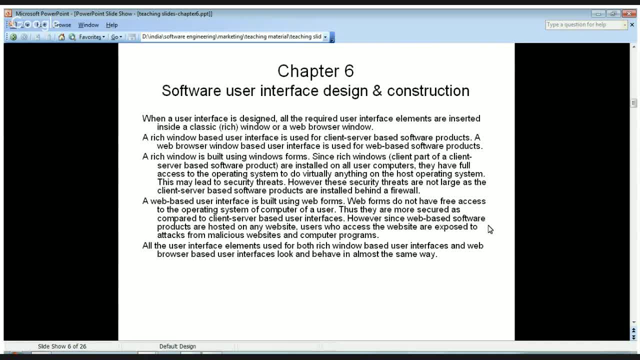 can do anything. so essentially it is risky. but generally the client server applications are used are installed behind the firewall, so outside people do not have access to these software products, so that way it is safe. and so even though they have they have, they are not secure. like uh, on the operating system it can do anything, but still 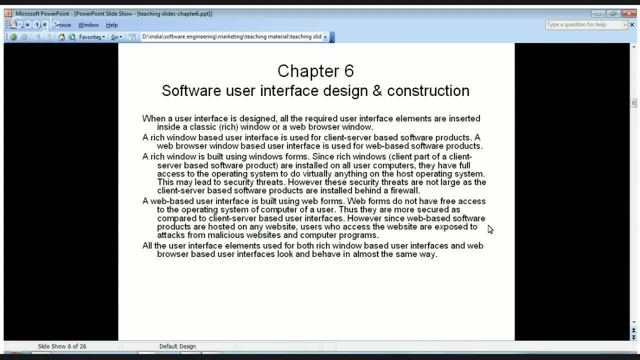 since only known people or a very few people will be using those products, so it is not a big issue. a web-based user interface is built using web forms. web forms do not have free access to the operating system of the computer of a user. thus they are more secured as compared to clients on this user interface. however, since 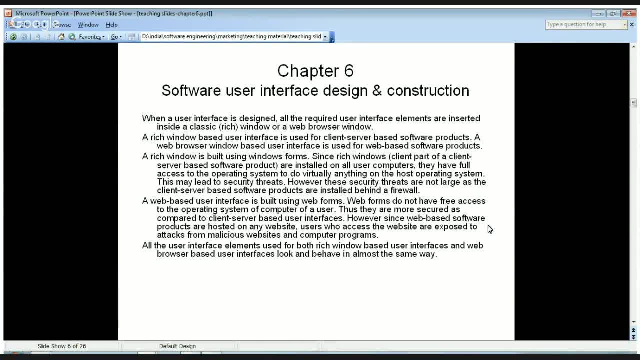 web-based software products are hosted on any website. users who access the website are exposed to attacks from malicious websites and computer programs, so web-based user interface uh are built using web forms and these web forms are more secure compared to which uh to to. you know this window forms because they see. essentially what happens is that these 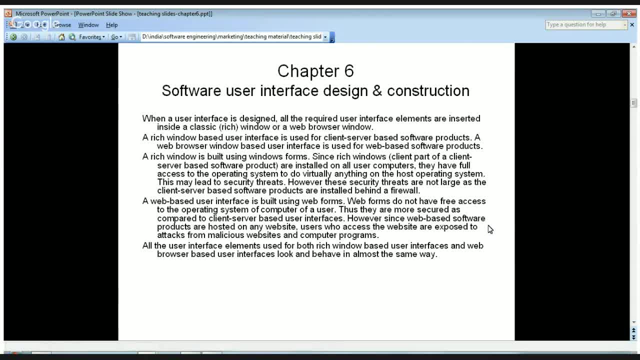 web forms or are inside of web pages. these web pages are are installed on a web server and when a user computer accesses a website installed on that web server, so those pages, web pages- will be shown on the user browsers. so generally that means the web forms are not installed on user computers, they are installed. 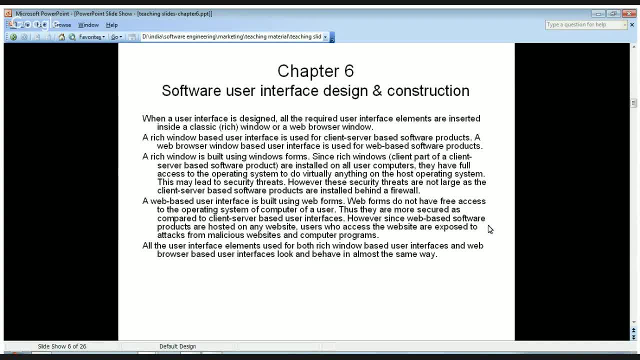 on the web server. so they, that way the user is safe. but the thing is, uh, since the user will be connecting to a web form, which is which we, which is inside a web page, using the internet connection, so through the username net connection, it is possible that. 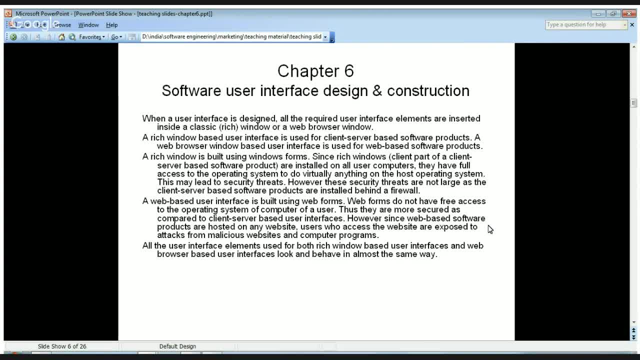 some, some malicious software product, say a virus may crawl in through this, this connection, and may infect the user completely. so for for that you need to ensure that the user interface you are creating in form of web pages. they are secure, like they are being, like. they are installed with the encryption, or very high encryption, to ensure the 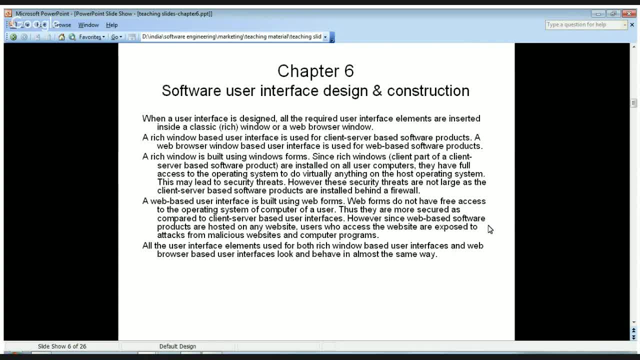 some malicious software product cannot read and write right inside those web pages when they are downloaded on user computer. all the user interface elements used for both which window base user interface and web browser based user interface- both can behave in the same way. so most of the user control elements. 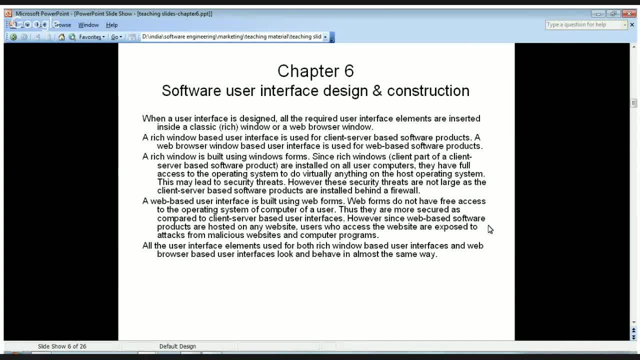 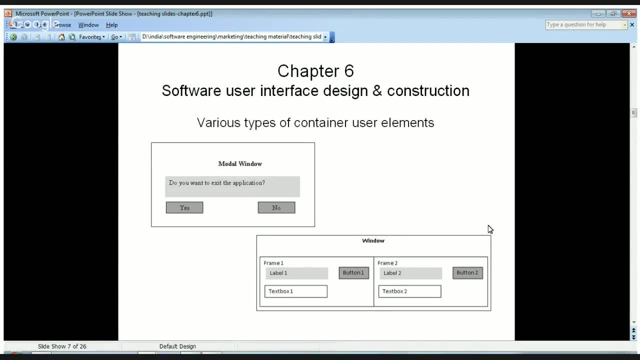 and for both the web browser user interface as well as rich window based user interface almost look the same and they do the same kind of stuff. now let us discuss these, the user elements. so here let us. it is displayed. two things are displayed. one is model window and another one is the frames inside a window. 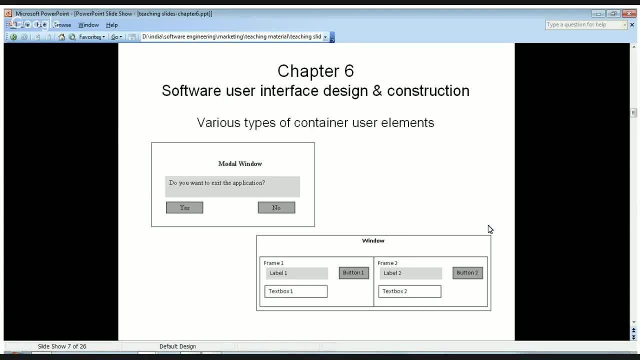 so model window is used when you you want the user to say: the user has clicked on something and it needs a decision to be made by the user, like the user wants to exit the application. so even though the user has clicked to click on some button to exit, but it still, the application may ask the user if the 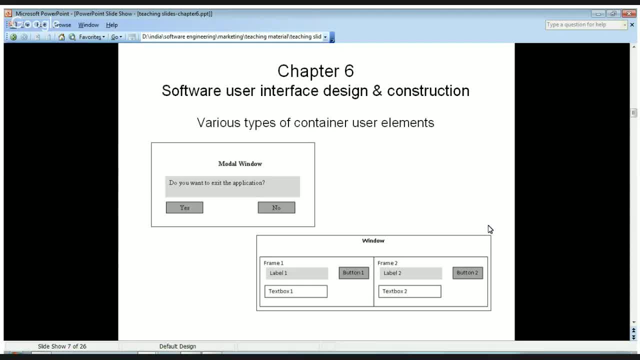 user wants to exit. so if the user clicks on yes button, then the user will exit from that application and if user clicks on no, then he will still be on the same application, connected the same application. so model windows are used for this kind of usage and then the frames are used to put together similar, similar user elements. 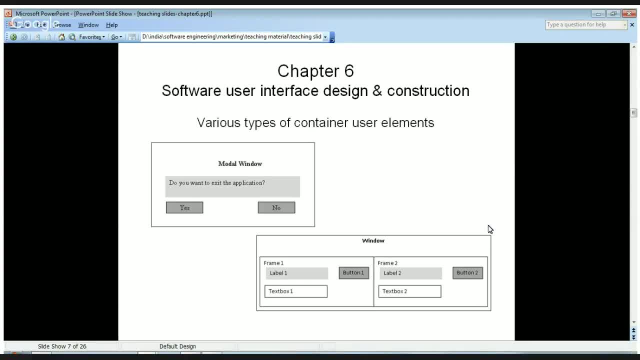 inside one frame and then another set of user elements inside another frame, like here it is shown: in frame 1 you have level 1, text box 1 and then button 1, and in frame 2 you have level 2, text box 2 and button 2. 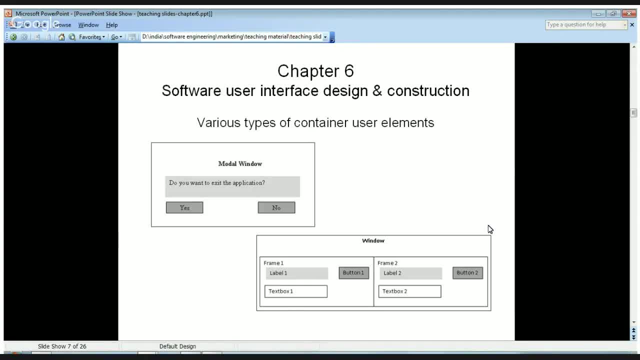 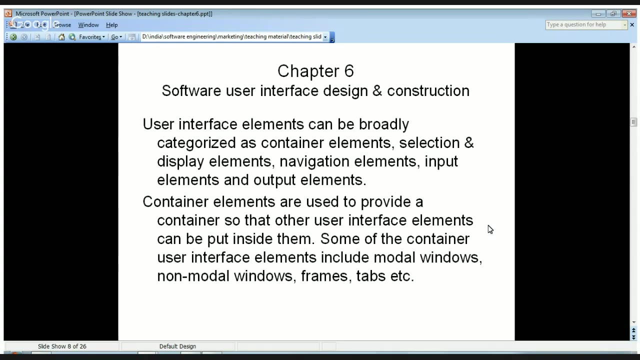 so essentially, the frames are used to separate out user elements on the same window. so here the you see these two types of container user elements. user interface elements can be broadly categorized as container elements, selection and display elements, navigation elements, input elements and output elements. container elements are used to provide a container so that other user interface elements can be put inside them. 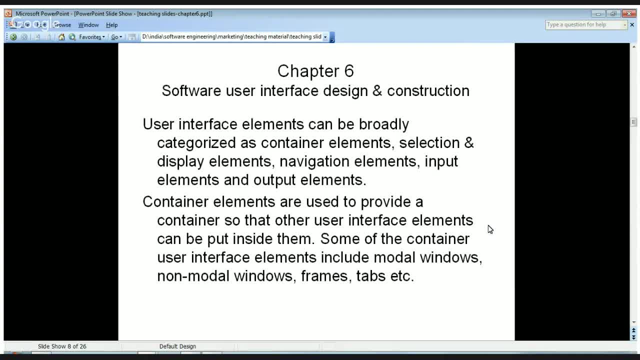 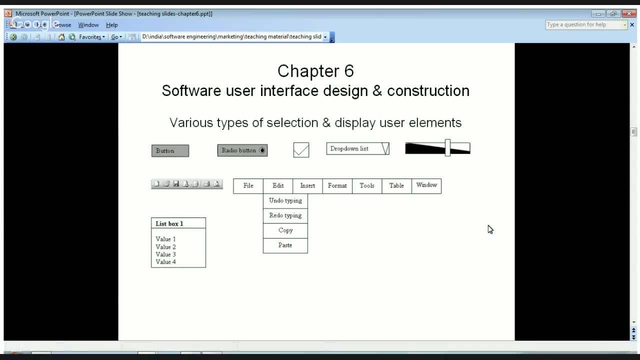 some of the container user interface elements include model windows, non model windows, frames, tabs, etc. so in the previous page you saw some container elements. now let us see selection and display user elements. so For making any selection or display these user elements are used. Like you use button, So button can be used for display or for selection. Then again radio button. In the radio button, like if you have two radio buttons to select option: yes or no. 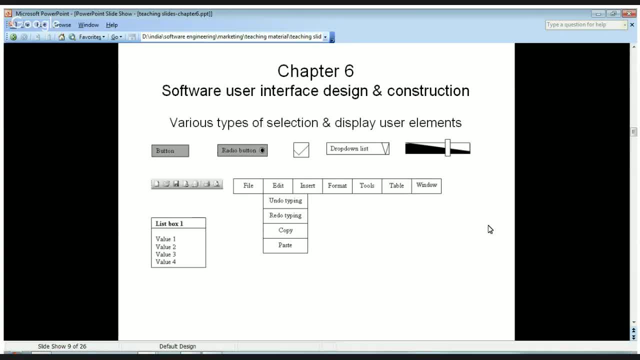 So one of them you select, So it is there. that means it can be used that way. Then you have check boxes. So check boxes also again. if you check a box, then that means you are selecting that option. Then we also use. we can have drop down list. So in the drop down list you can see a lot of options. When you click on the drop down list you can see a lot of options. 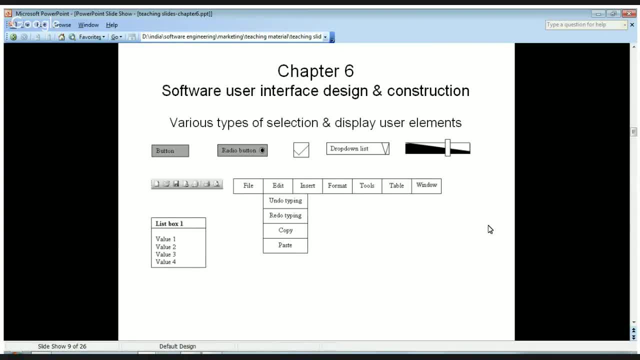 If you click on the arrow button tab on this list, the list will be displayed and all the options will be available. So this is how you can use the drop down list. Then you can have a. you can have an icon tab where you can have. you can put the control buttons on a tab and when a user clicks on any of those icon buttons, the program will execute and it will navigate to that part of the software product. 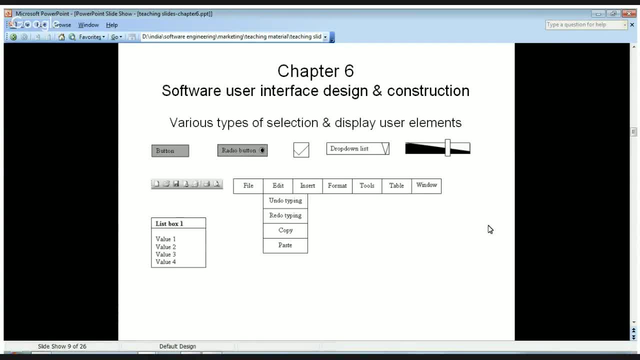 Then you can have menus. you can have drop down menus. So using menus you can navigate, you can select which part of the software product you want to see. like in a typical Microsoft Word program you have edit menu. So when you click on the edit menu you will see some sub menus like undo typing, redo typing. 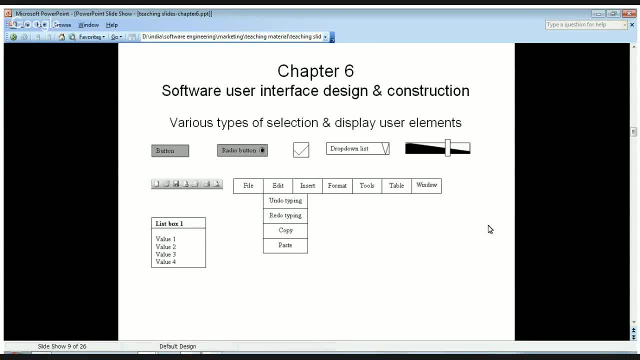 Copy, paste, etc. So using one of those sub menus you can do your work. Then you also can have list boxes. So a list box shows a lot of options. So you can select any of the options and the software product will perform the option which you selected. 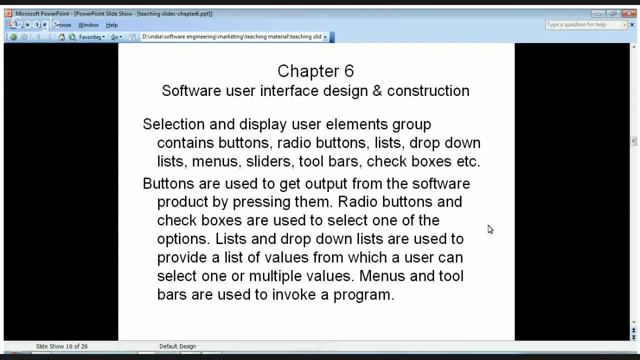 Selections and display user elements contain buttons, radio buttons, lists, drop down list, menus, sliders, toolbar, check boxes, etc. Buttons are used to get output from the software product by pressing them. Radio buttons and check boxes are used to select one of the options. 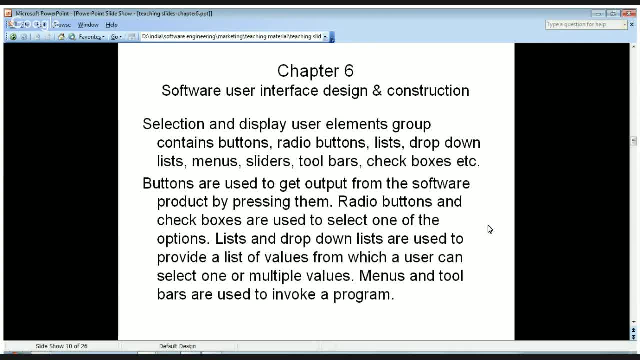 lists and drop down lists are used to provide a list of values from which a user can select one or multiple values. toolbars are used to work a program. so this is how you can use these user control elements. you can put them on when you design a user interface and then the business logic you can. 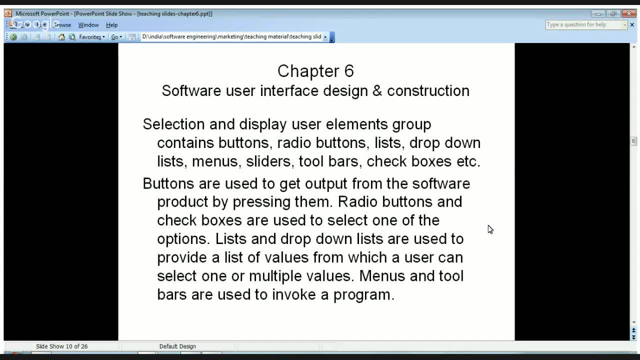 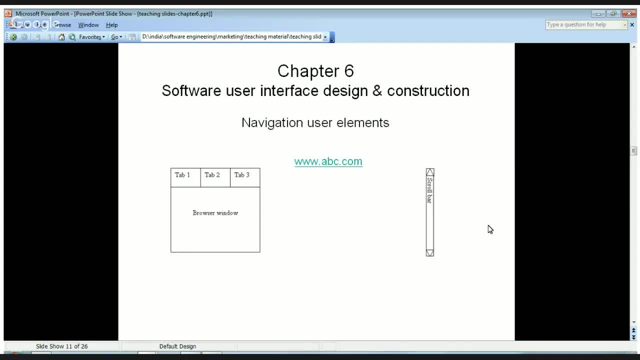 write down business logic later for doing the work, computing which is required. then we can have navigation user elements like links like here. you can have wwwabccom and when a user clicks on this link so the user will be navigated to that web page, then we can. you can have tabs. you can insert tabs inside your web form or window form. 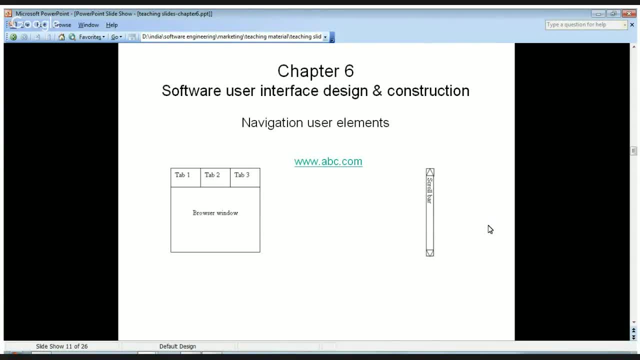 and on each window, on each tab, there will be a window attached and on that window, all the, it will work like a complete window. nowadays, if you see the, the, any web browser, any web browser contains a lot of tabs. like you, you can create one. you can. 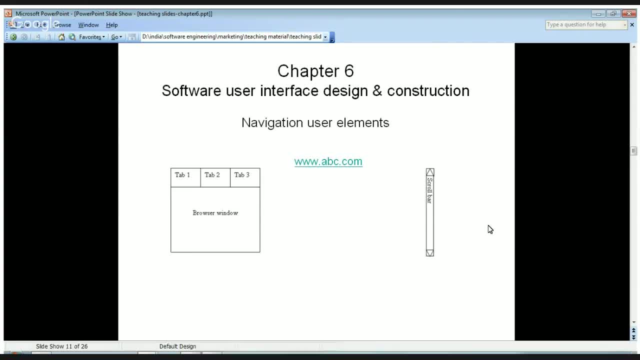 start one tab and you can have one web page. then you can create one more tab and you can have another web page. so this is how you can use tabs, and then you can put a scroll bar on the right side of any web page so so that user can scroll down or scroll up on a on a page. navigation, user element groups. 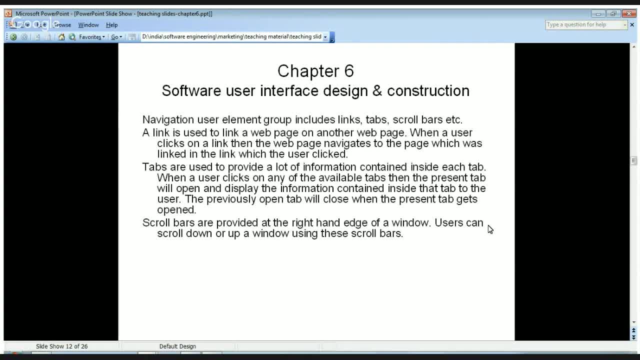 include links, tabs, scroll bars, etc. a link is used to link a web page on another web page. when a user clicks on a link, then the web page navigates to the page which was linked in the link which the user clicked. tabs are used to provide a lot of information contained inside each tab. 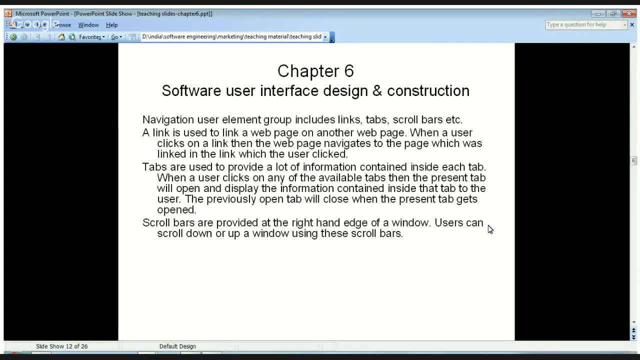 when a user clicks on any of the available tabs, then the present tab will open and display the information contained inside that tab to the user. the previously opened tab will close when the present tab gets opened. scroll bars are provided at the righthand edge of a window. 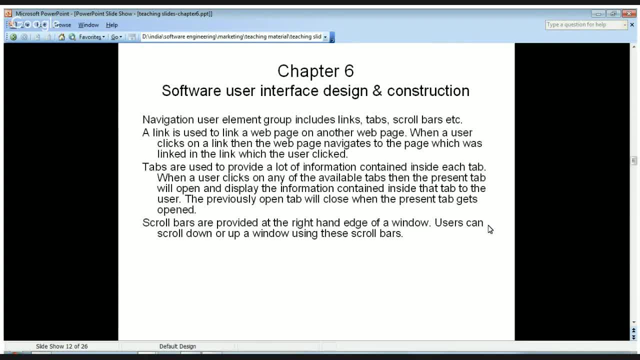 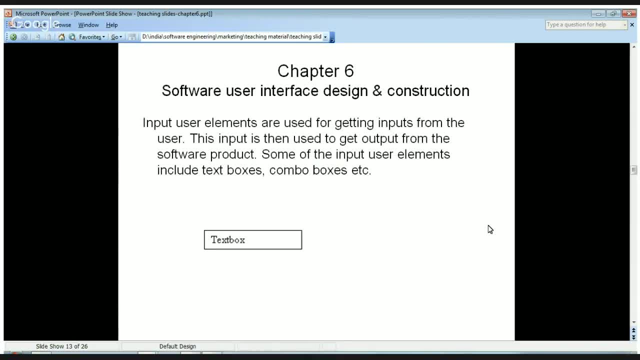 user can scroll down or up a window using these scroll bars. now come to input user elements. essentially we can have text boxes for providing input. so if you you put a text box on when you design a user interface, so when the software product runs, then in that text box 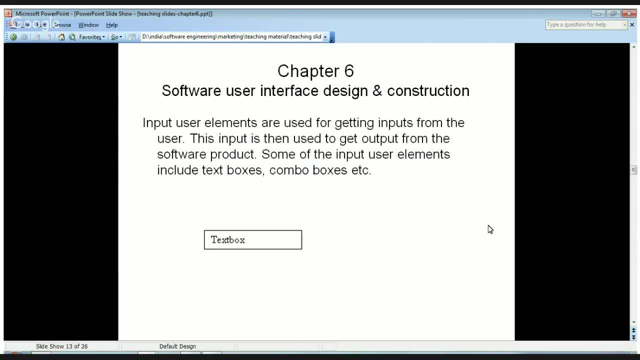 the user is supposed to provide some input and when the user clicks on some button to process, then whatever input provided by the user will be taken, will be processed and, by the business logic and coming to output user elements and, like you, can have output in form of label or tooltip or 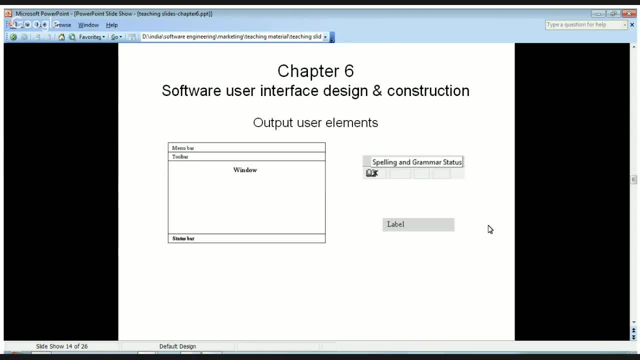 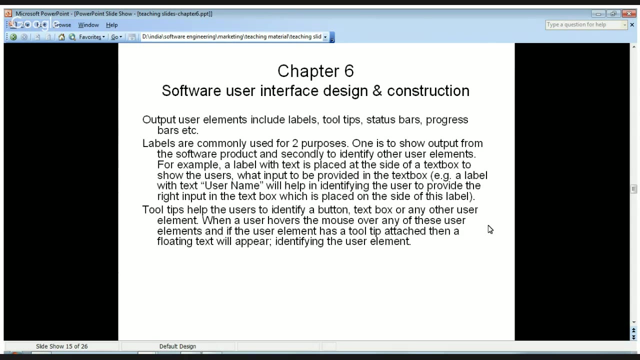 status bar, etc. so the user elements output. user elements are used to provide the output from the software product to the user so that the user is able to process the output. the user can can see and get that information. output user elements include labels, tooltips, status bars, progress bars, etc. labels are commonly used for two purposes. one is to show 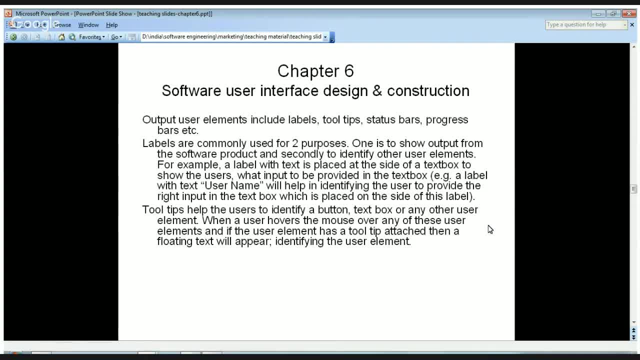 output from the software product and secondly, to identify other user elements. so labels are used for two purposes: one is to show output and another is to identify other user elements. for example, a label with text is placed at the side of a text box to show the users what input to be provided in. 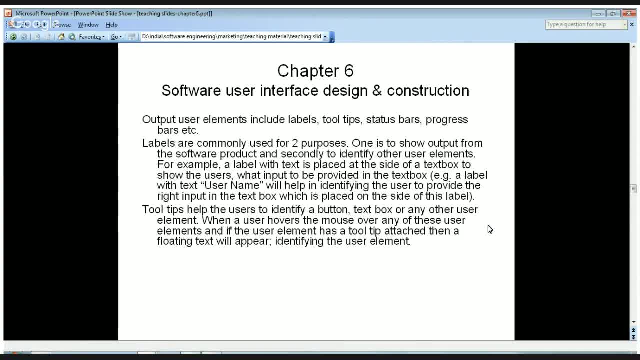 the text box. for example, a label with text username will help in identifying the user to provide the right input in the text box which is placed on the side of this level. tooltips help the users to identify a button, text box or any other user element when a user hovers the mouse over any of 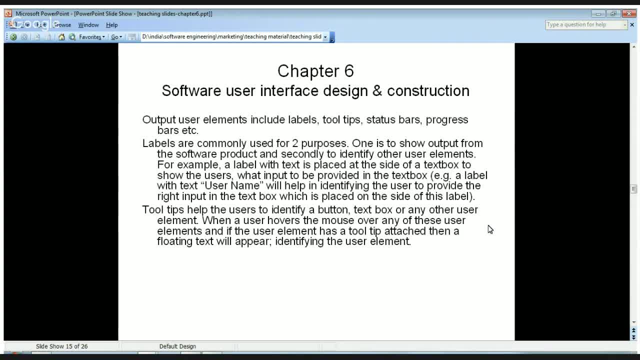 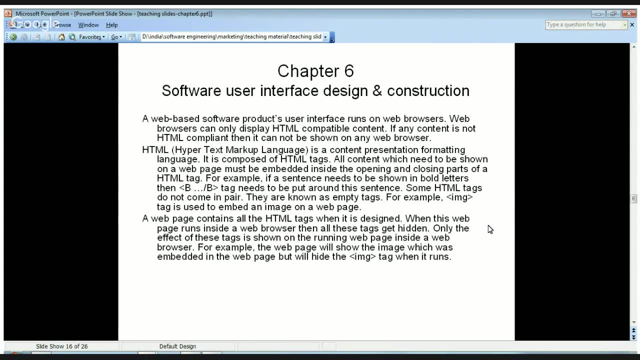 the elements, and if the user element has a tooltip attached, then that floating text will appear identifying the user element. so that was all about user elements. now we will come to the next one, the html. a web-based software products user interface runs on web browsers. web browsers can only display html compatible content. if any content is not html, 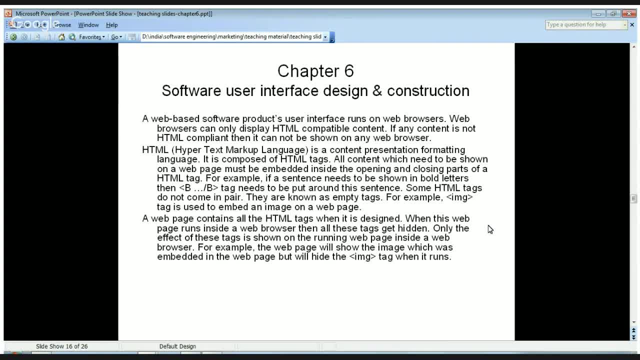 compliant, then it cannot be shown on any web browser. html- html is a short for hypertext marker. markup language is a content presentation formatting language. it is composed of html tags. all content which need to be shown on a web page must be embedded inside the opening and closing. 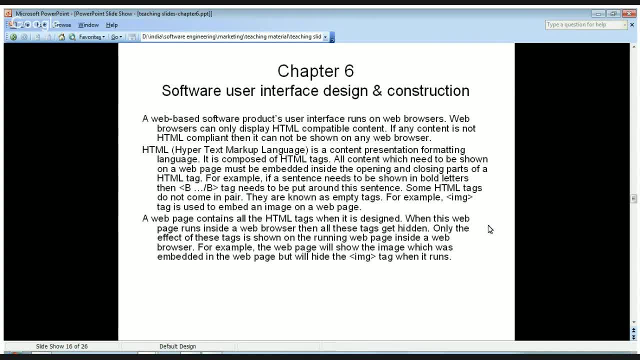 parts of a html tag. for example, if a sentence needs to be shown in full letters, then opening braces b and then a slash and closing slash b and closing this tag needs to be put around this sentence. so when this is done, then then the the letters which were put inside this html tag will be shown in bold. 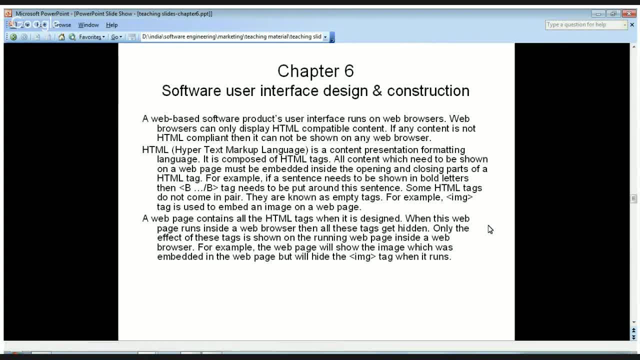 some html tags do not come in pair. they are known as empty tags. for example, uh. for image there is a html tag base: img closing. this tag is used to embed an image on a web page. a web page contains all the html tags when it is designed. when this webpage runs inside a web browser, then all these tags get hidden. 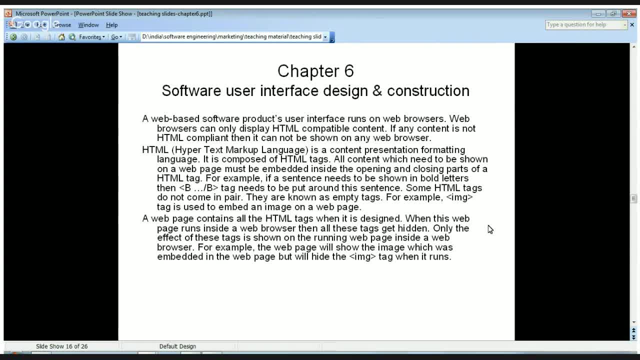 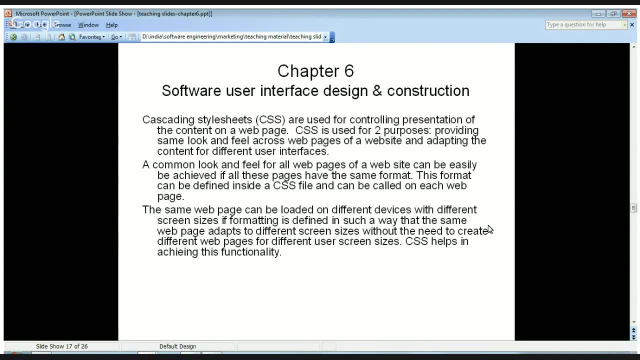 only the effect of these tags is shown on the running web page. inside a web browser, for example, the web page will show the image which was embedded in the web page, but will hide the img tag when it runs. we also have cascading style sheets along with the. 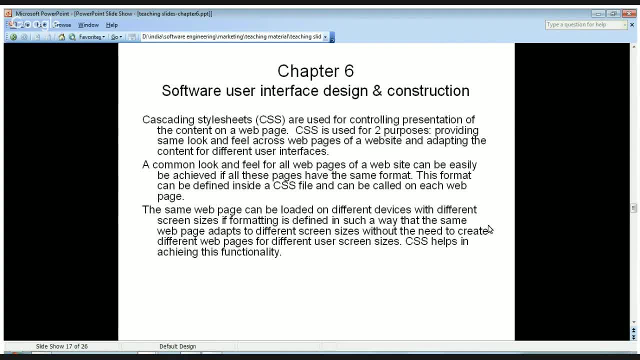 HTML and why cascading style sheets are used. let us see. cascading style sheets are used for controlling presentation of the content on a web page. so, even though it is similar, but we use cascading style sheet because of two purposes: one is providing same look and feel across web pages of a website and second, adopting 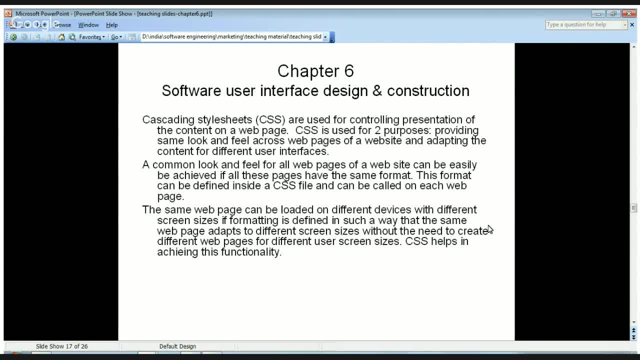 the content for different user interfaces. for example, we have a website which can be shown on any any web browser, like, say, you have a mobile headset and you have a laptop, so the screen size of these two are very different. the laptop screen size is very large, so it can. 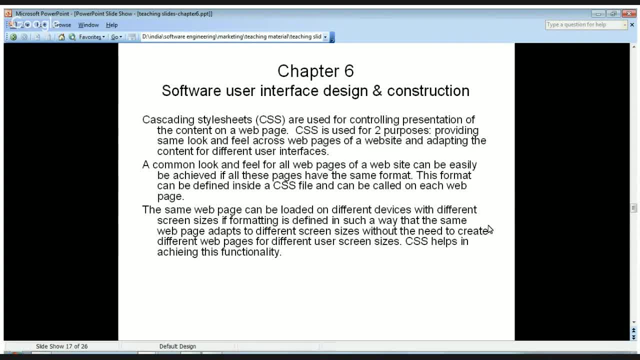 display the complete web page, but the same web page you want to display on a mobile device, then you cannot display everything on a on the screen of a mobile device because it is very small. so you may not- you may want to- to hide some of the information of the in. 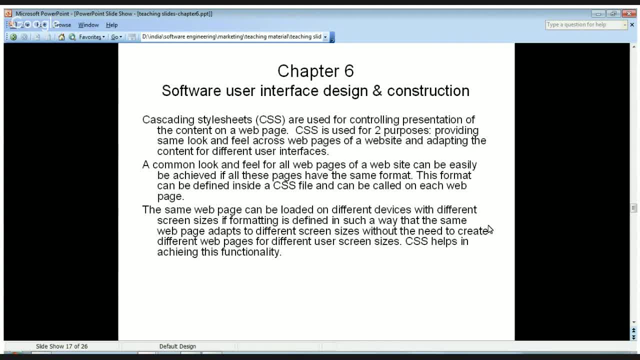 information of the page. and secondy, you want to show them in the texture. you want to reduce the size of different parts of the window so that it can fit inside this small screen of the mobile device. so in that case you will use cascading style sheets. so you will create two sheets for these purpose, one for a. 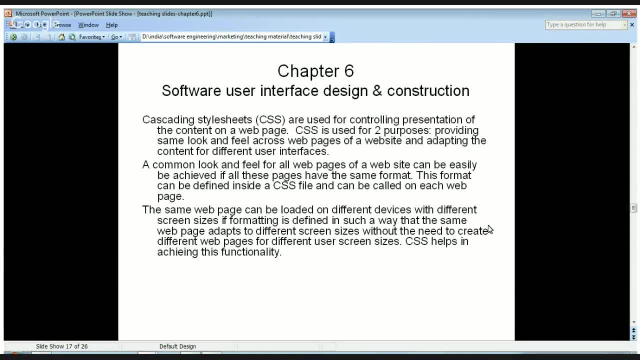 normal window or laptop and another style sheet for the smaller screen of a mobile device. Similarly, the other purpose of style sheet is like what you can do: you can create a file containing the formatting, all the formatting you want to do. you create a style sheet file and you 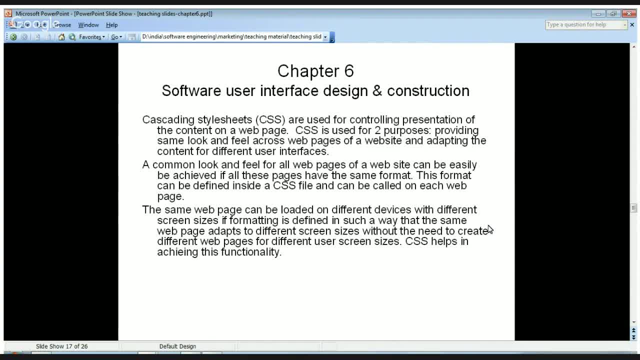 save it and then, on the, when you create the web page, on the web page you can call this file, this style sheet file and all the formatting which you defined in that file. you can save that file and will be applicable on the web page on which it is called. So this is how. 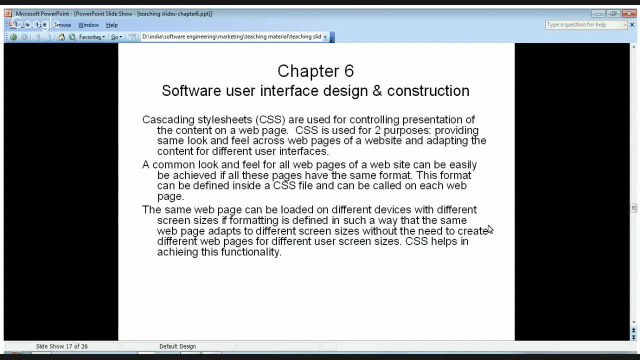 style sheets are used. A common look and feel for all web pages of a website can be easily achieved if all these pages have the same format. This format can be defined inside a basketing style sheet file and can be called on each web page. So this file, like you created. 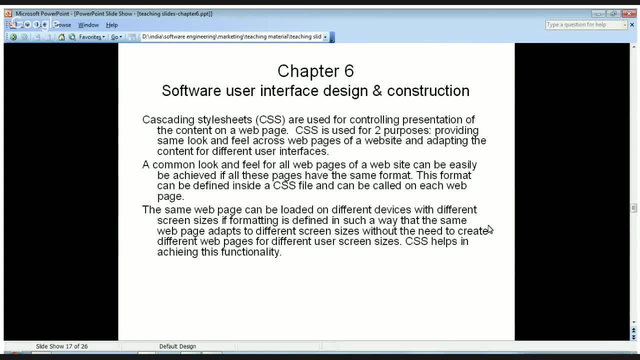 a style sheet file file. like abccom, you can create a style sheet file and you can now install it on your website and you can see a file which is called style sheetcss and on each say you have five web pages for a website. So on each web page you can call. 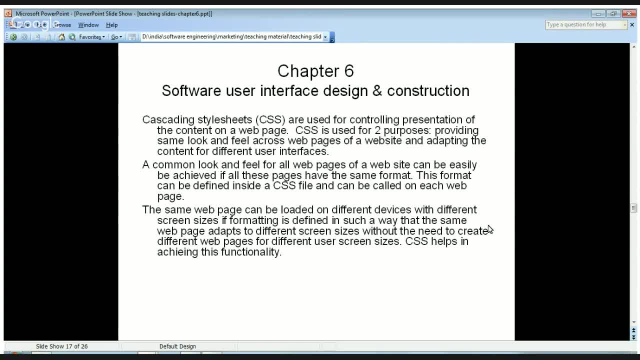 this file. So when user hits your website and sees your web pages, he can see the same format for all the other web pages, because the style sheet, the way in which the website is created, is different from what is in other web pages. So when you create and paste your 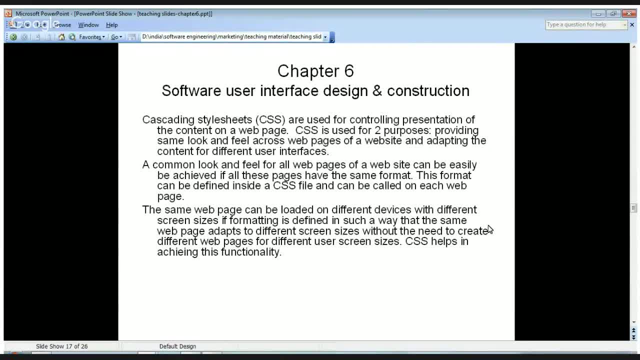 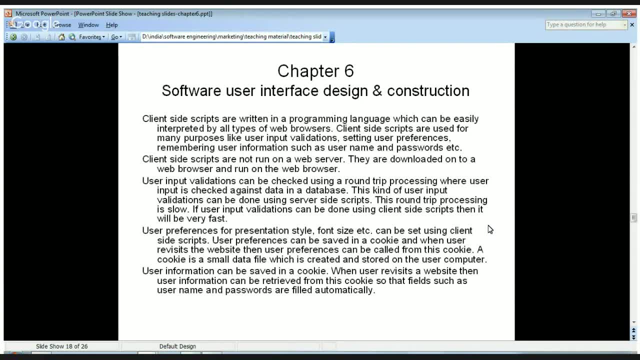 you use is the same on all these web pages: client. now, now we are coming to to writing the code which is used for user interfaces. they are known as client-side scripts. client-side scripts are written in a programming language which which can be easily interpreted by all types of web browsers. 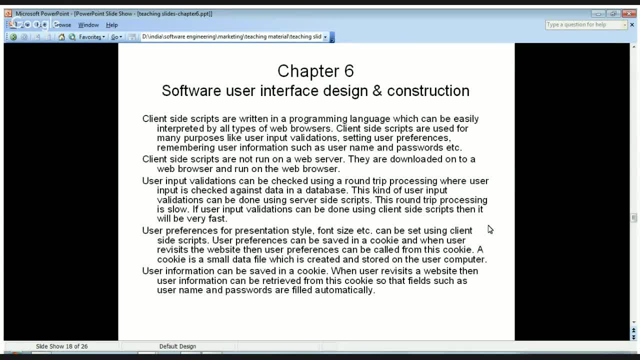 client-side scripts are used for many purposes, like user input, validations, setting user preferences, rewriting user information such as username and password, etc. so client-side scripts are used for these purposes. then client-side scripts are not run on a web server. they are downloaded onto a web browser and run on the web browser. 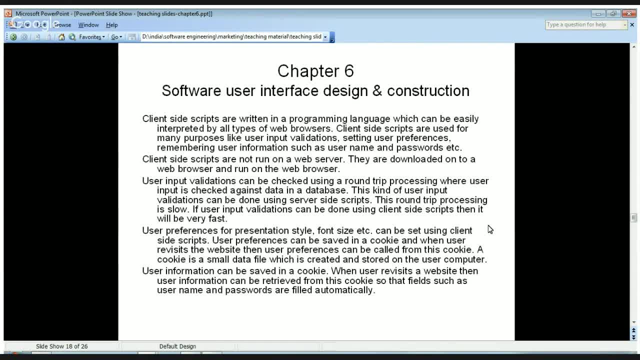 so, essentially, the client-side scripts are actually downloaded on the web browser. they do not run like. if a web page has a client-side script and a user browser connects to this web page, so that script will be downloaded to the web browser and if it and it will run inside the 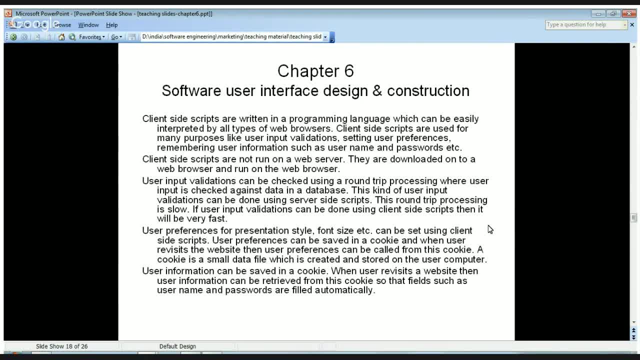 web browser. all the web browser has capability to run client-side scripts, so it will run, and then, uh, the content out of this script will be shown to the user. user input validations can be checked using a round trip processing, where user input is checked against data in a database. so 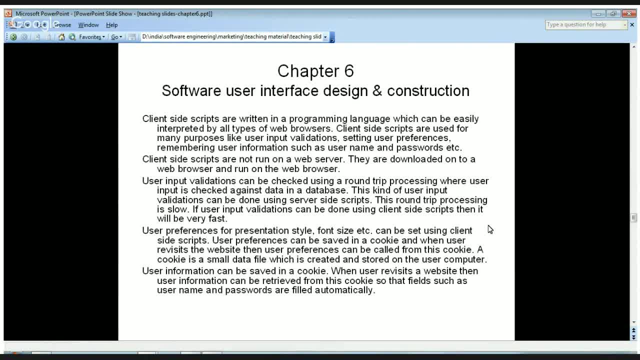 user input validation like a you like, say for a password field. uh, you want to ensure that the user- uh only a password filter should be- should accept only a length password field length of four character to eight, correct. so you need to put this validation, otherwise the user can write any uh. 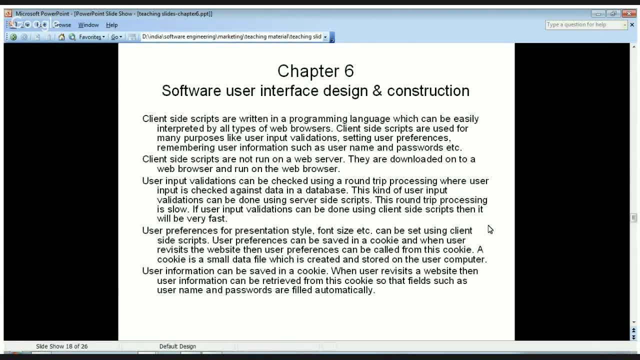 can define, can write a password of any length. so definitely you need to provide this validation so that users are restricted to use a specific length of password field. and it can be like validations can be done using uh, using checking the values, the input values of the user in a database. in that case, 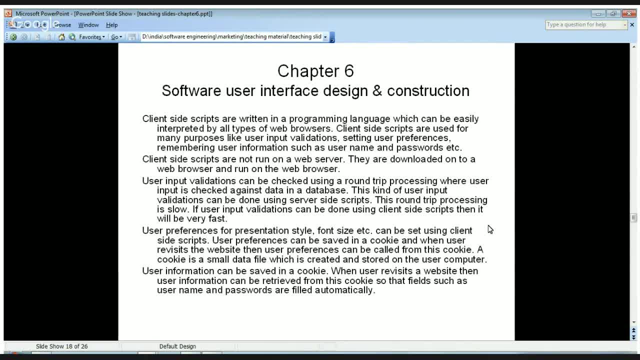 when the program runs. so it will go through the business logic and then it will go to the database and see some value in the database and then come back whether this say you: on the login page you provided some password and it needs to be checked. so this password you you put as input will be checked in the database. it is correct. 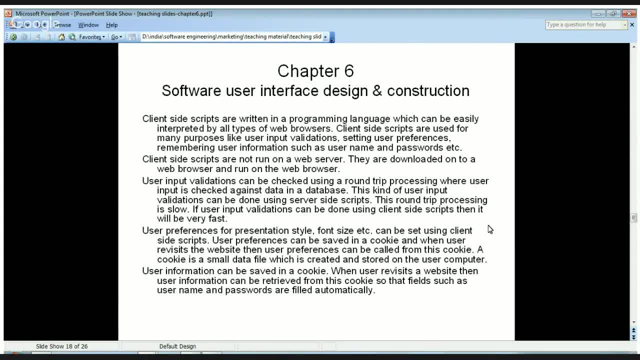 and then it will come back and say that okay, this password is correct and you can log in, otherwise it is incorrect. then you will not be able to log in. so this kind of processing is done, uh, through what is known as a server side script, where you can check the values in a database. but this kind of checking will take time. 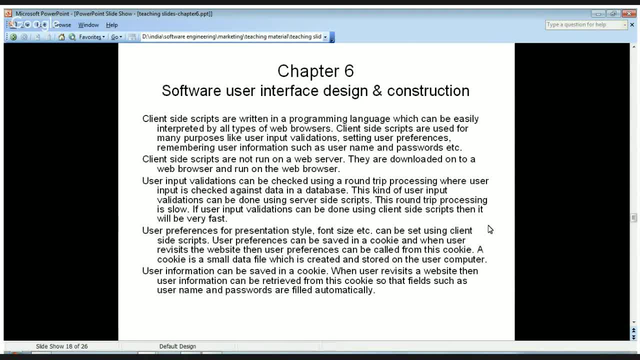 like it will go up to database and come back. so, instead of that, what you can do, you can do this validation on the client side itself, like you can write a client-side script and you can do the validation. so, even though there are some restrictions as to what kind of validations you can do on the client, 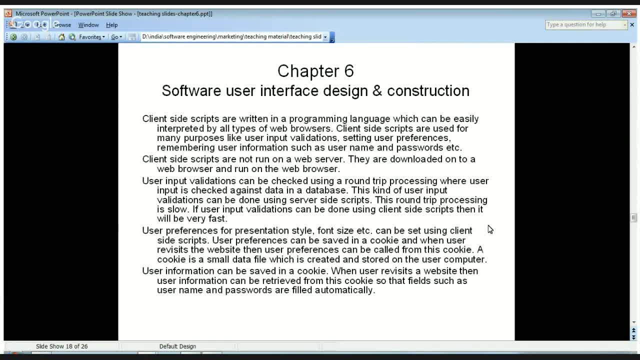 side, but it is better because, uh, this is kept, will run on the browser itself, so it will be very fast then. user preferences for presentation style, font size, can be set using client-side scripts. user references can be saved in a cookie and when user really visit the website then user preferences can be called from this cookie. 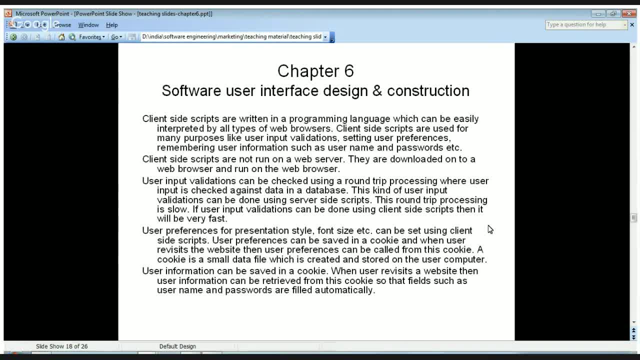 a cookie is a small data file which is created and store on the user computer. suppose you want to set user preferences for presentation style, font size, or even you want to remember some user information, so you can use a cookie. so the software, the client side, discreet, will write a cookie on your computer and save the information, the information inside. 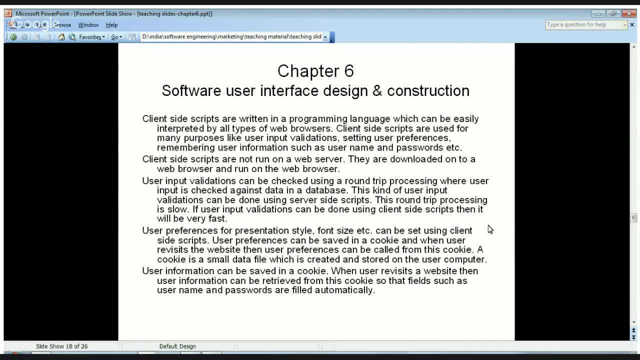 this cookie. the first time you'll be the website. the next time you you will read this website, then your the client had escaped. I will try to find out if there is a cookie already installed, already saved on the computer. and if it is there, then it will read that cookie and then it will come back. and then it will it will. 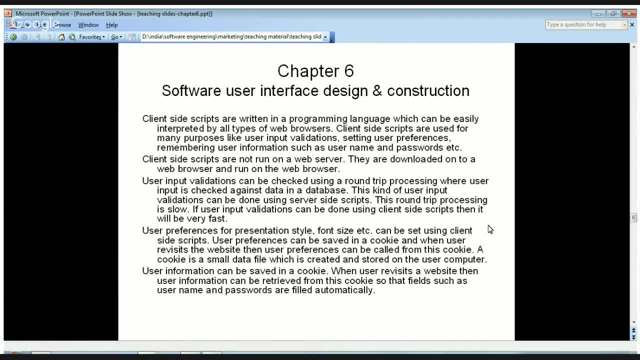 show to the user like the user preferences for a website, so those will be set and the user will see the content in in his script in his style. presentation is time. user information can be saved in a cookie. when user re-visits a website then user information can be retrieved from this cookie so that fields such as 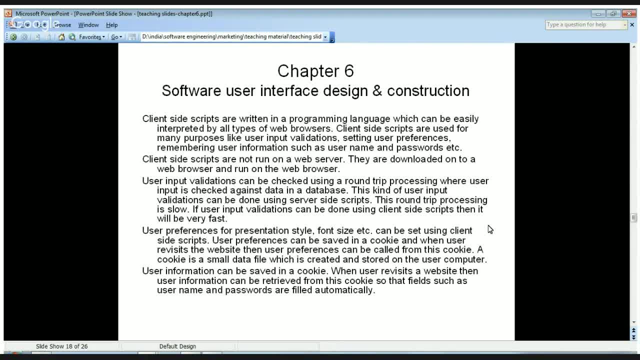 username and password are filled automatically. so automatically filling some input elements like the username and password can be done through a cookie, like if the information is available about the user in a cookie like username and password, and the user re-reads the website, then the transit escape will read that cookie and then finds the information of username and password. 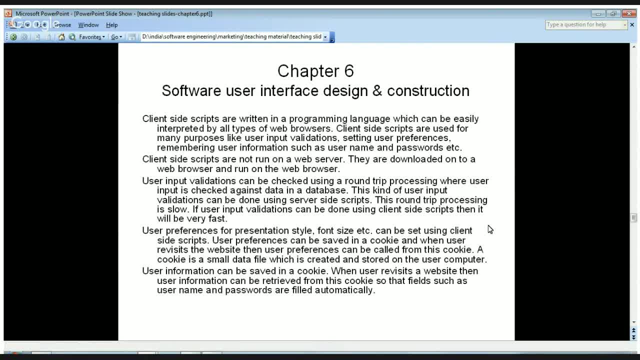 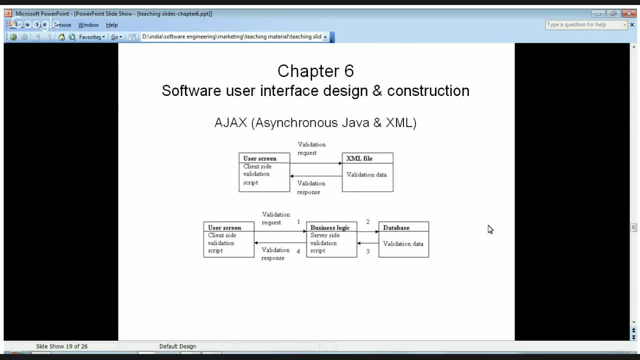 and then fill can fill the this information on the web page automatically. okay, now one technology which is used for user interfaces is known as ajax. ajax is short for asynchronous java and xml, so the the earliest implementation of ajax was there used to be client side validation script and there would be a xml file. 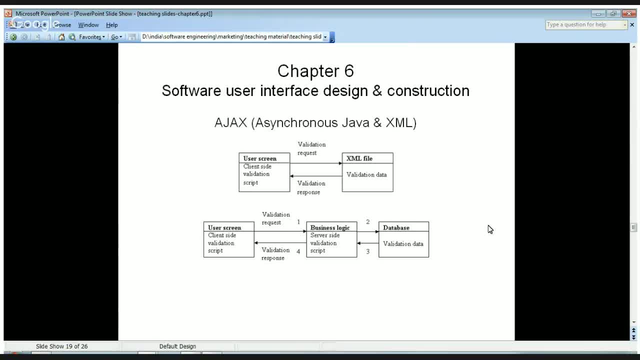 where some validation data will be there. the validation data will be read in the xml file and then validation can be done for a user, for a for on a web page. so this was the earliest interpretation. later ajax was modified and now it is it can do also. yeah, okay, now this is the therive prompt, which is also can be used to chaotic. 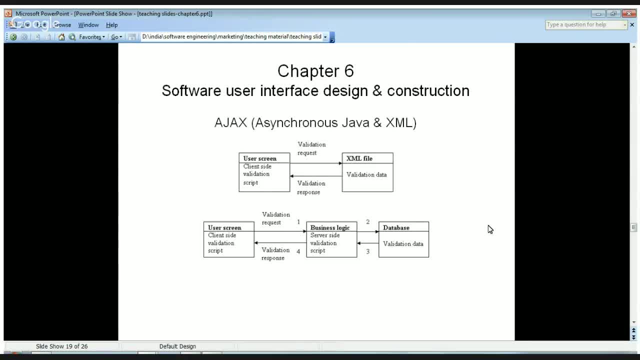 enabled meetings, but it is very useful because it allows you to visualize the data, whether the data is time-restricted, the data is vale generated through the interface of 얼�ax or just utilizing the interface as it is now. such function can help things in the web, for example if you have a client-side validation script. 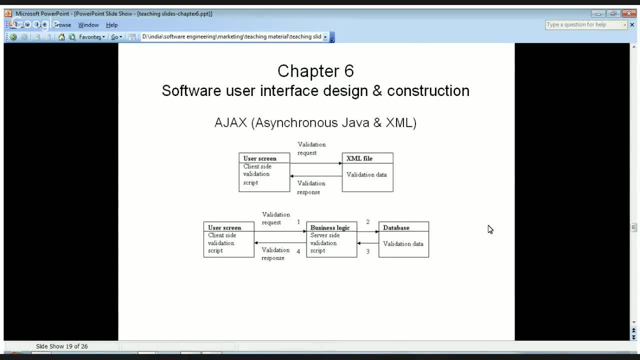 validation response will be given to on the user screen, so it will go all through this process. and Ajax is used in many instances, like on web page, if the user needs to do some registration. so the user needs to fill a lot of text boxes. so in some cases it is actually useful, like: suppose you have- you have- a username. 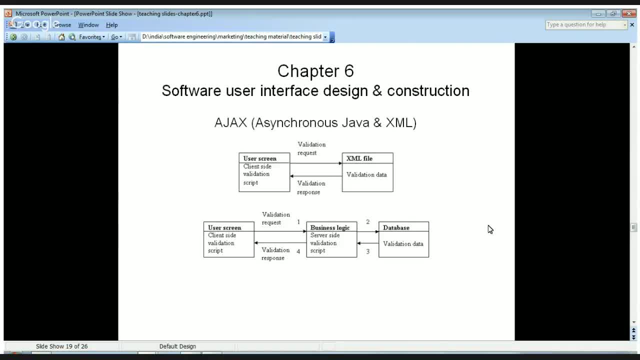 field you need to provide a username to get registered on the website and you provide the username and password and your information etc. and then you click the button. when you click the button to process your information for registration, and suppose the username you put is already taken by somebody else, so that 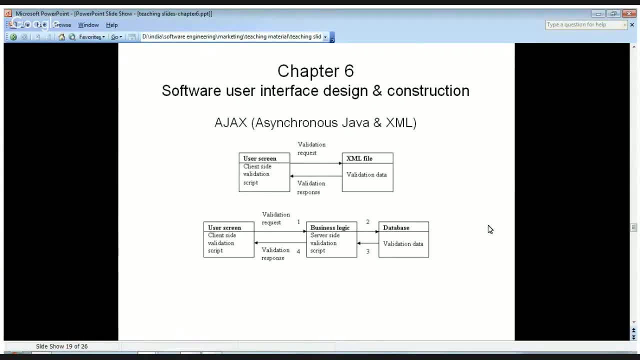 means when your information, registration information, is processed. so in the database it will be seen that already the username you provided is not available and you need to provide another username. so, since this is the web-based product, so what happens is the moment your web page navigation happens to all the information provided on the. 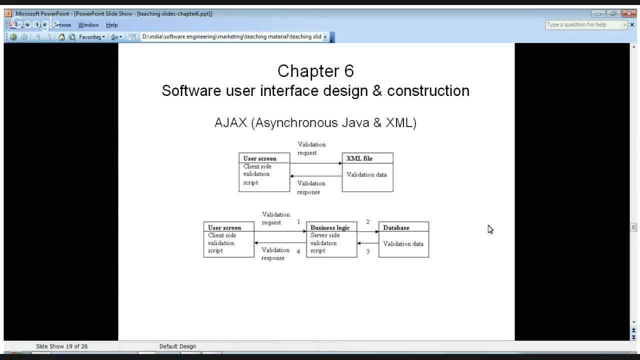 web page is lost, since in the database nothing will be written because the username is not available. so again the web page will come back to the user and say that the username is not available. please provide another username. so this way it is a lot of problems for the. 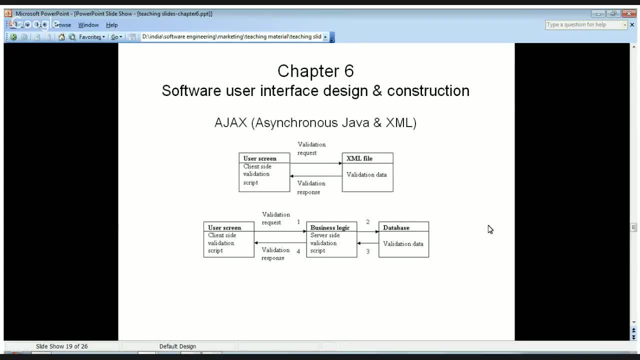 user, like you, can try another username and if it again it is already taken. then again we will have to provide all the information necessary to provide a very specific user about registration. so Ajax helps in this kind of scenario. what it does is when the user provides the username, some input on the username and then the user 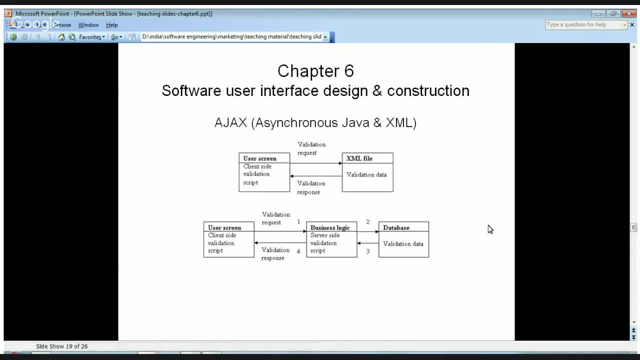 moves to some other other field on that web page. so the moment he moves event might move move of event in invoked and using this moving work event, the the username field, information will be taken and it will be processed in the business logic and in the database. it. 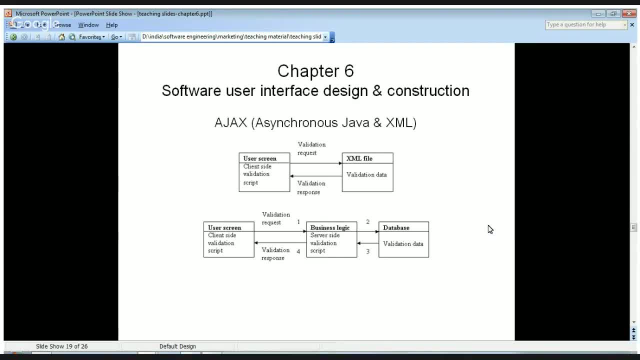 will be checked. if it is available, then it is fine. if it is not available, then it will come back and then it will show this from: this username is not available and please provide another username. so that way the user user is will again employed another user name. 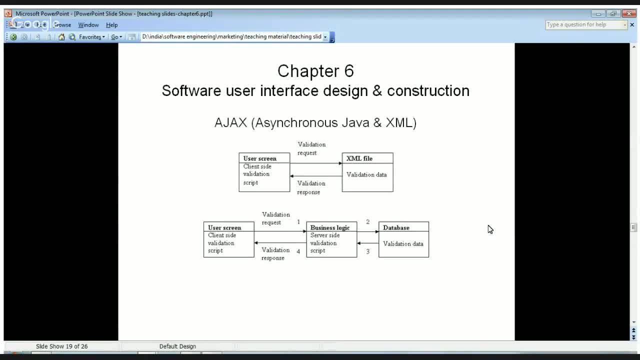 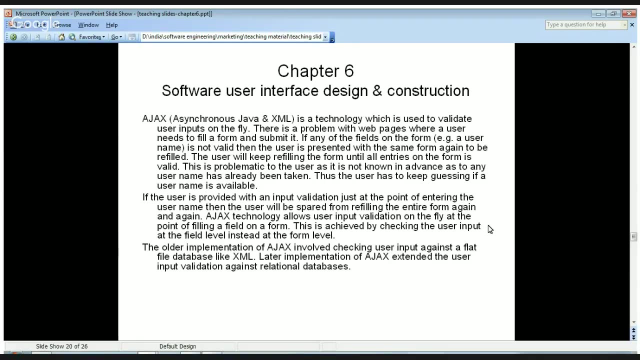 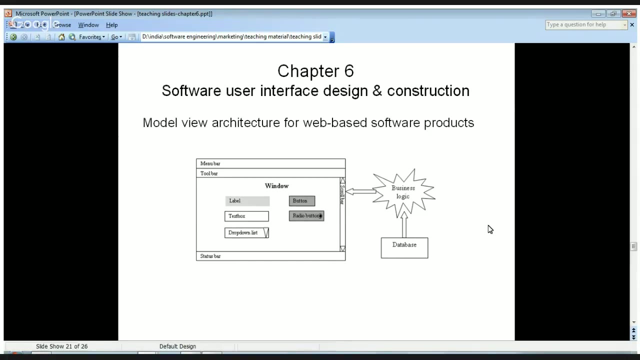 but he will be saved from the fact that other fields he has not. he does not have to write again, again and again. so this is how it works. now coming to to model view architecture and some other kind of architectures or user interfaces for database software products, generally a lot of software. 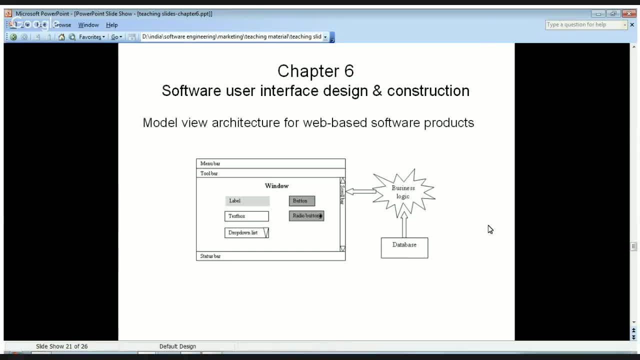 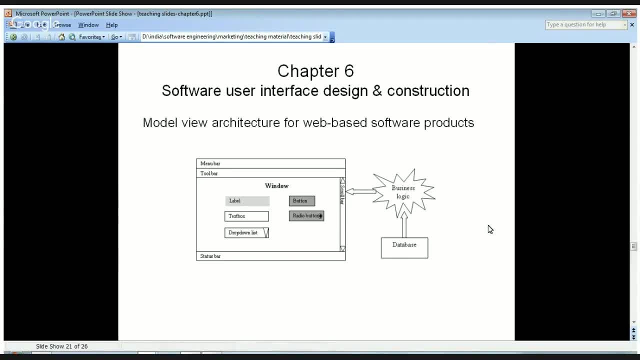 process and then the flow, data flow- will happen and the business logic will run and the database will be connected, some information will be obtained that will be written in the database or something, and then your process is complete. so this is how model you architecture works, what we also have. 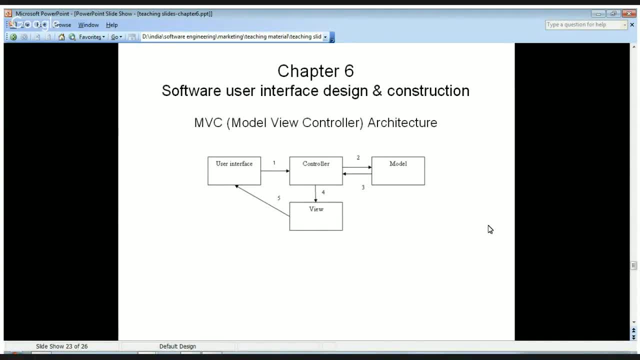 another architecture which is known as model view controller. so in the model view controller you have three parts. in the earlier one we saw in the model view controller you have three parts. in the earlier one we saw in the model view which is similar to model controller, which is somewhat like a topic, but this one- 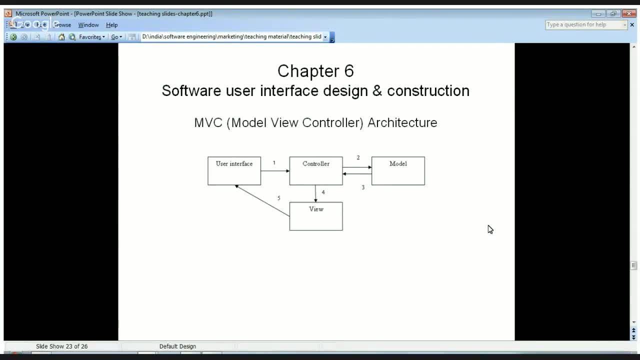 is very privacy free, so we are going to use three eleven part and which is much more. other is the data planning which we will never talk to, your lectern outlet, which is model v architecture. there were only two parts, like the view, which is, which is which is shown on the user interface, and model model means the business logic. 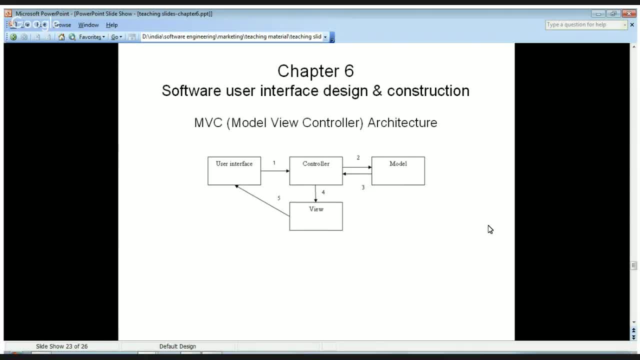 but in model view controller we have one more element: the controller. so here you have the user interface and then you have the controller at the model and some input is provided on the user interface. it passes to the controller. it does not part. the passes pass directly to the model. 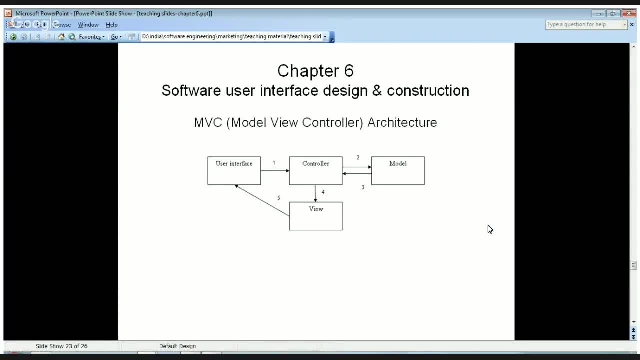 it passes to the controller, then controller will find out, find out if model has to do something. so it will ask the model to do some processing. the model will do some processing and will come back and point that information to the controller. then controller will decide if some view has to. 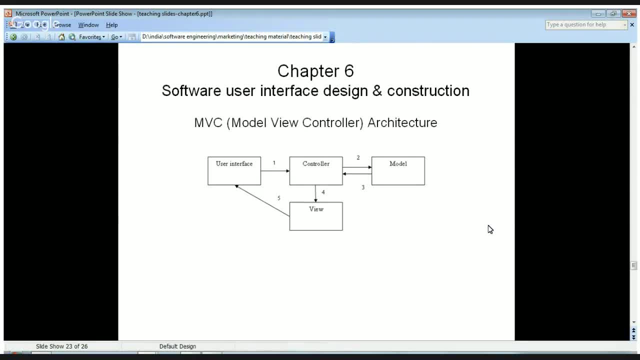 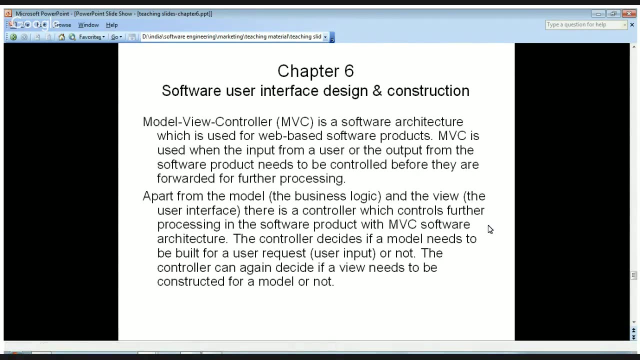 be created, and if some view has to be created, it will create, and then this view will be available at the user interface. so this is how model view controller architecture works. model view controller, or in short mvc, is a software architecture which is used for web-based software products不用. 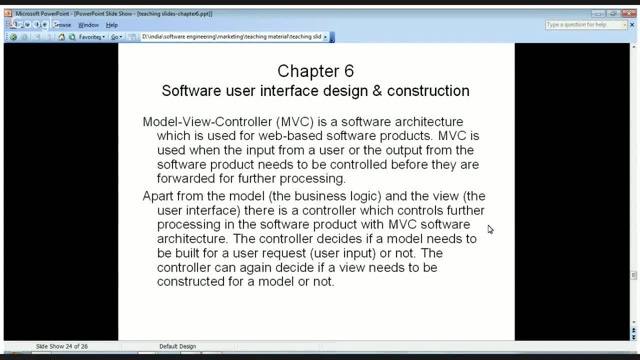 is used when the user from a user or the input from the user or the output from the software product needs to be controlled before they are forwarded for further processing. apart from the model- the venus logic- and the view- the user interface, there is a controller which 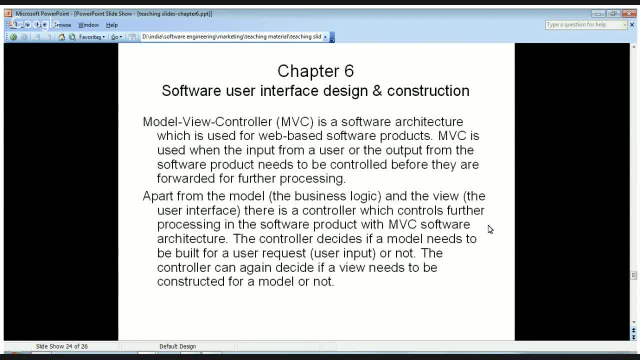 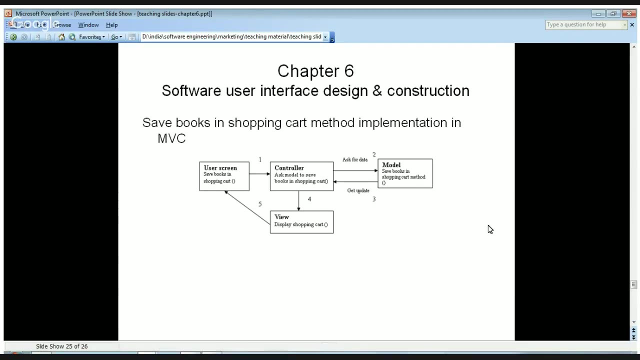 controls further processing in the software product. with mvc software architecture, the controller decides if a model needs to be built for a user request or not. the controller can again decide if a view needs to be constructed for a model or not. one example of this mvc architecture: 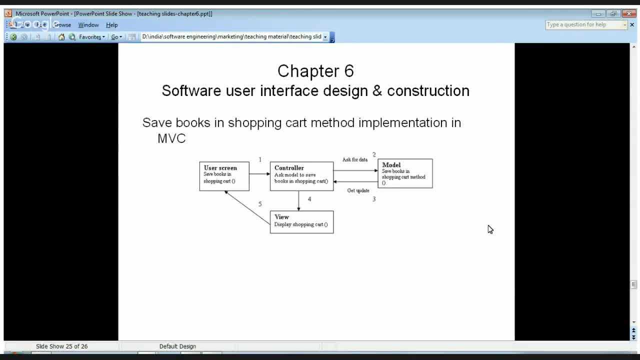 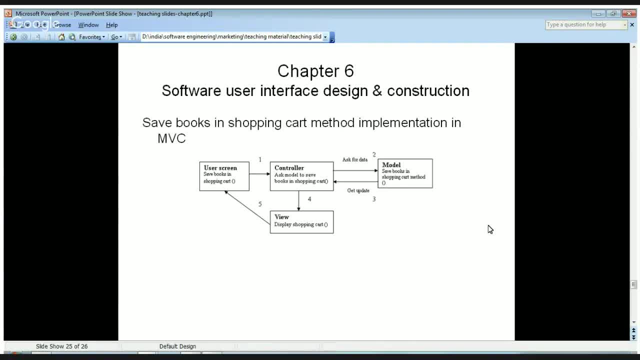 at the stage of checkout, all the books which you you selected will be shown and you want to purchase them. then you proceed further in the meanwhile, like when you are browsing, so you browse one book. if you do not select, you go to the next book and you read some information about that book if you like then 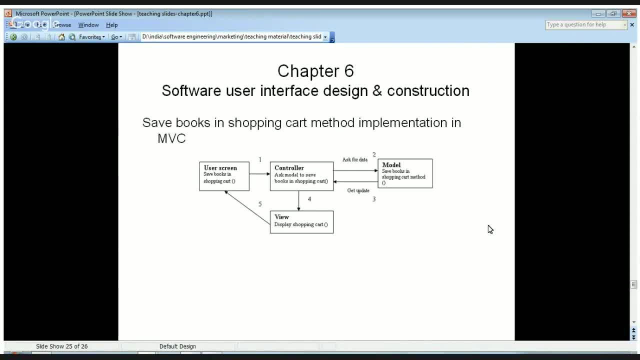 you select this book, you go to the next book again, you read information about that book. if you don't like, then you move to the next book. so books which you like, so they go to your shopping cart, and the books you do not like, they do not go to your shopping cart. so here a controller is actually controlling how the view 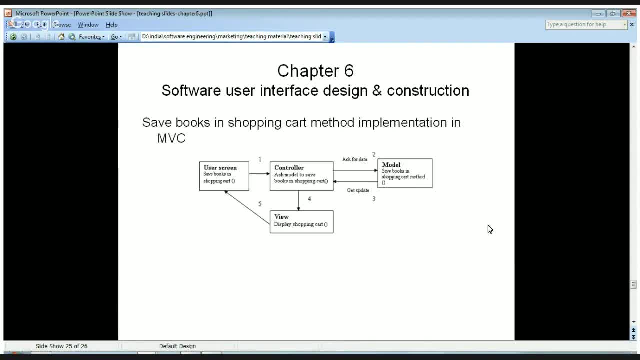 you are seeing should be constructed any at what stage, like when you are browsing from one book to another book. some information will be kept in memory and it will not be shown to the to you, but when you click a check checkout button, then all the selected books will be shown on a web page. 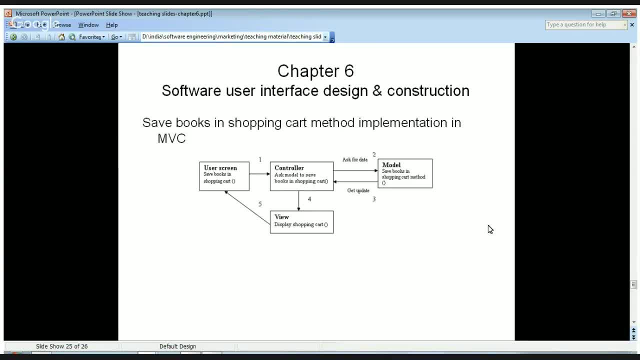 so that means the view, uh, the view which you you want to see, depends on the controller. so for this, this website for books- here is one example shop- like you want to save books in in a shopping in the shopping cart, so the controller will have some method like ask model to. 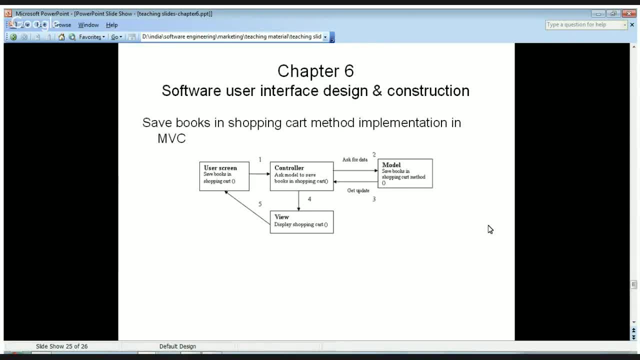 save books in the shopping cart and it will ask for data. the model will save books in the shopping cart, it will have a method to do that and it will provide output to the controller and then the controller will. since you want to check out, when you want to check out, then the display the shopping cart. if you are not, 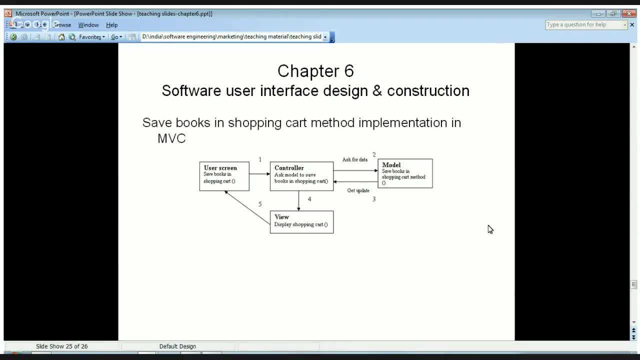 checking your you. when you are not clicking on a checkout, then you will keep browsing. the moment you click on a check out button, then it will create a view to display the shopping cart and this you will be displayed to the user. so this is how this MVC architecture works. the MVC architecture can be.